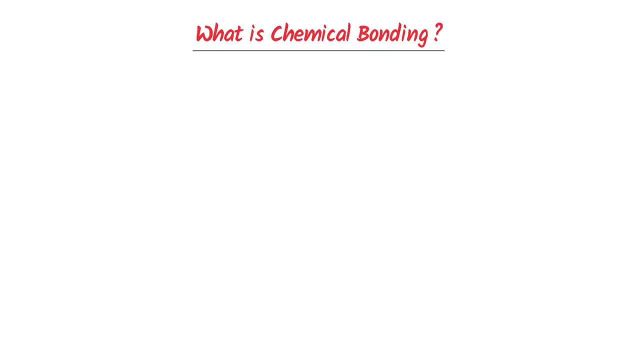 What is chemical bonding? Well, to learn the concept of chemical bonding, consider daily life examples like salt, common sugar, like glucose and water. We know that salt is made from two atoms, like sodium and chlorine. glucose is made from three atoms, like carbon, hydrogen and oxygen, while water is made from two atoms like hydrogen and oxygen. 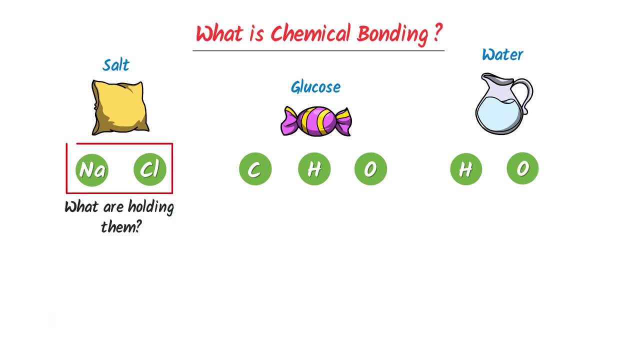 Now let me ask you: what are holding sodium and chlorine to form salt, What are holding carbon, hydrogen and oxygen to form glucose, And what are holding hydrogen and oxygen to form water? Well, the answer is simple: Attractive force: hold sodium and chlorine to form salt. Attractive force: hold carbon, hydrogen and oxygen to form glucose. 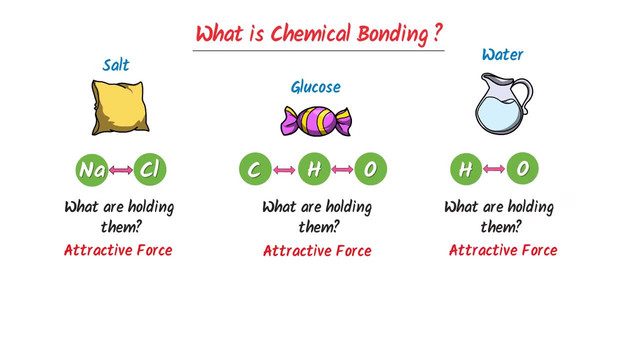 Attractive force hold hydrogen and oxygen to form water. Now listen carefully. In chemistry, the attraction force between atoms, ions and molecules to form a chemical compound is called chemical bond. Let me repeat it: The attraction force between atoms, ions and molecules to form a chemical compound is called chemical bond. 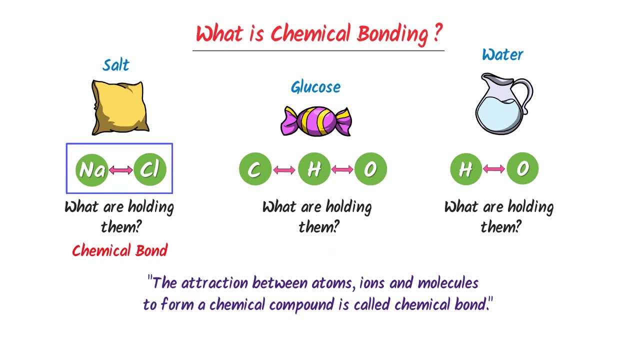 Therefore we say that chemical bond exists between sodium and chlorine to form salt. Chemical bond exists between sodium and chlorine to form glucose. Chemical bond exists between carbon, hydrogen and oxygen to form glucose. Chemical bond exists between hydrogen and oxygen to form water. 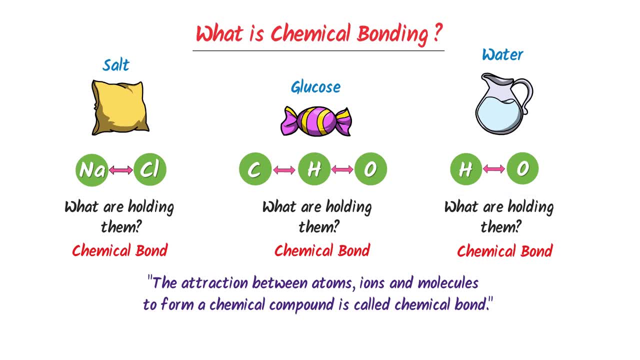 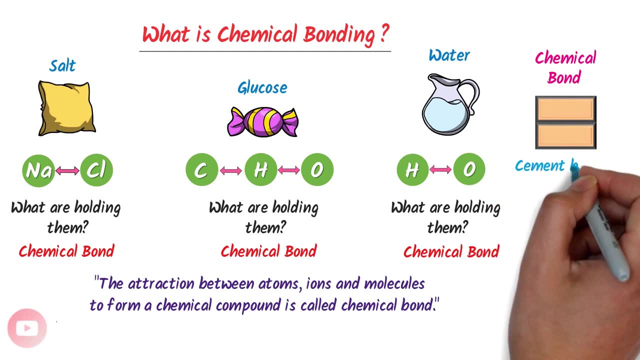 Thus we say that it is the chemical bond that is making everything around us. In simple words, we say that chemical bond is just like cement that holds two bricks together. Therefore, note it down that chemical bond is the attraction force. Chemical bond exists between atoms, ions and molecules to form a chemical compound. 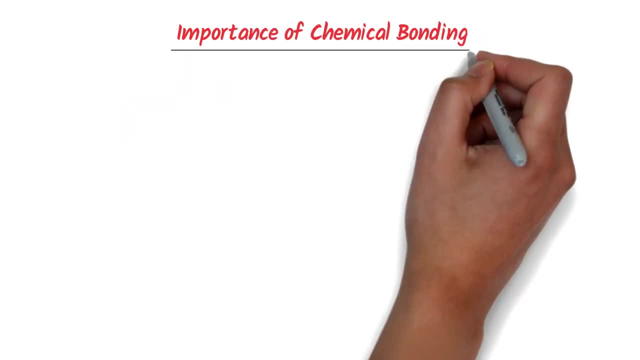 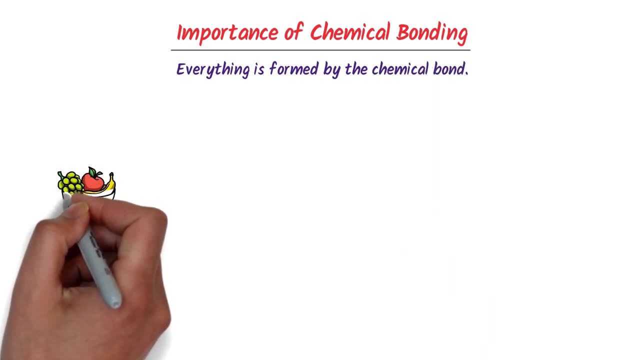 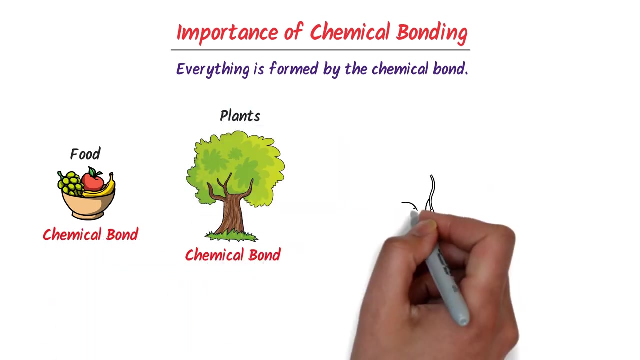 Now let me teach you what is the importance of chemical bonding. Well, everything in the universe is formed by the chemical bond. For example, the food we eat is made by the chemical bond. The plants we see around us are made by the chemical bonds. 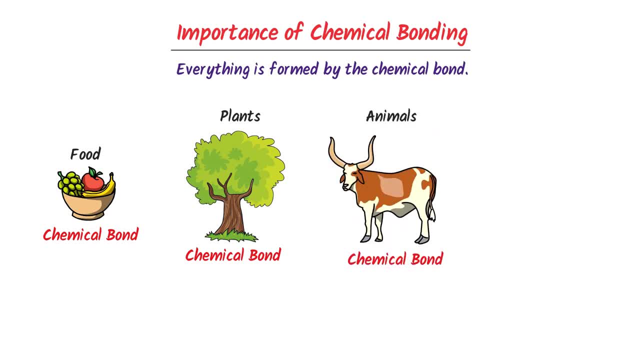 The animals we see are made by the chemical bonds. All the material we use in our daily life, like iron, plastic, etc. are made by the chemical bond. Thus, remember that it is the chemical bonding between atoms that form everything in the universe. 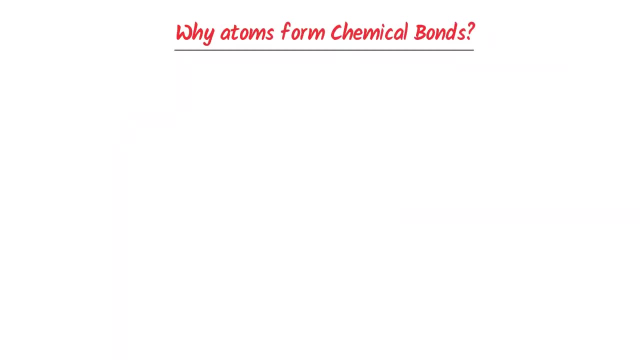 Now you should also learn that. why atoms form chemical bonding? Well, atoms form chemical bonding in order to lower its energy and get stability. Now let me ask you: how can we measure the stability of an atom? There are two simple rules. 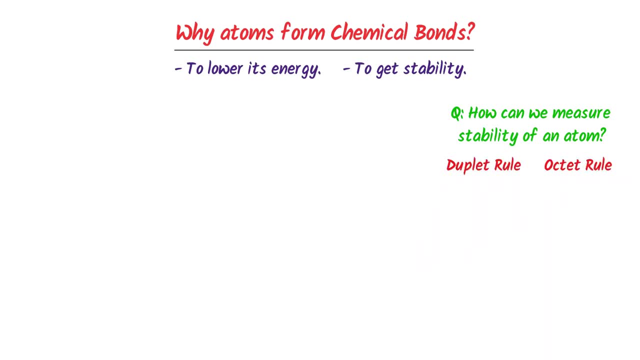 The duplet rule and the octet rule, which measure the stability of an atom. According to duplet rule, if two electrons are present in the last shell of hydrogen and helium, then they both are considered stable atoms. According to octet rule, if eight electrons are present in the last shell, 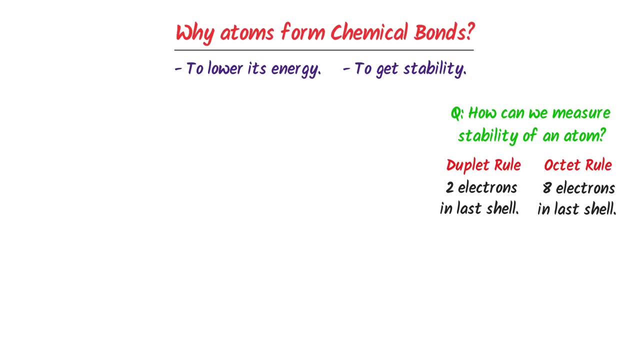 then atoms are considered stable atoms. For example, consider sodium and chlorine. We can see that in the last shell of sodium atom there is only one electron, while in the last shell of chlorine atom there are seven electrons. Now sodium will lose this one electron. 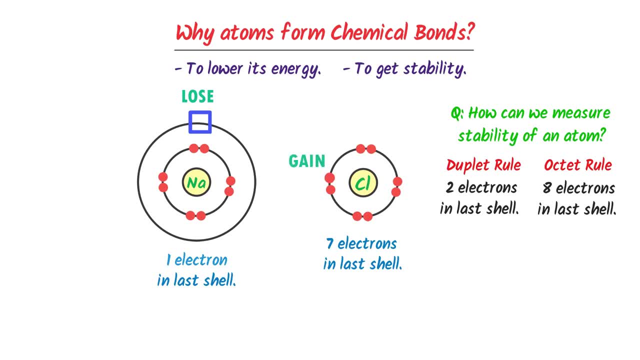 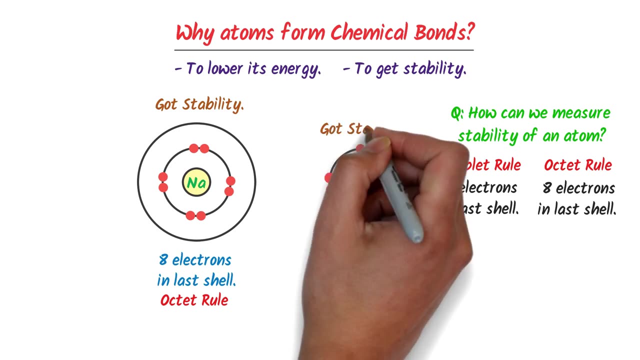 And chlorine will gain this one electron. So we can see that there are eight electrons present in the sodium atom And there are also eight electrons present in the chlorine atom. So the octet rule of sodium is completed And the octet rule of chlorine is. 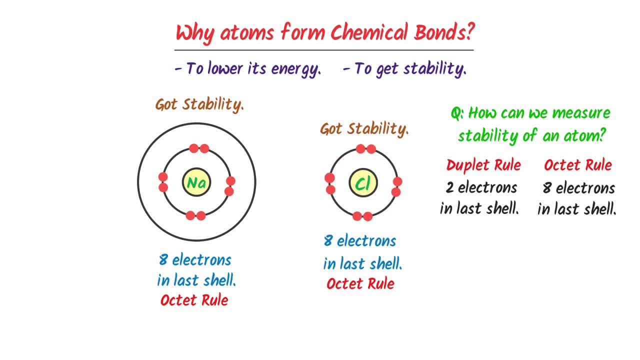 green is also completed. Thus, by losing and gaining electrons, they both form a chemical bond. Here let me teach you one bonus point: In order to lose and gain electron, suitable condition should be provided to an atom. Otherwise, atom will neither gain nor lose an electron. 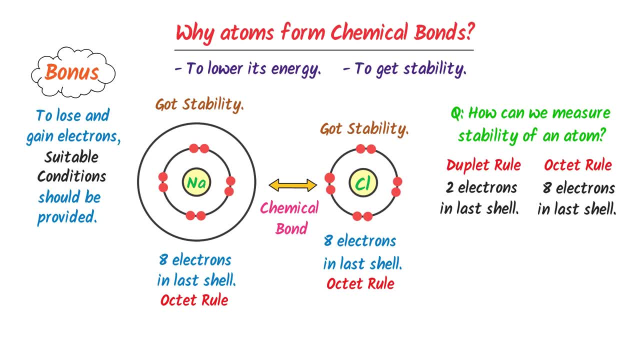 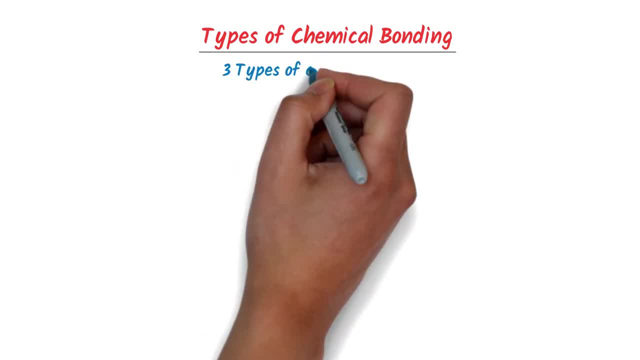 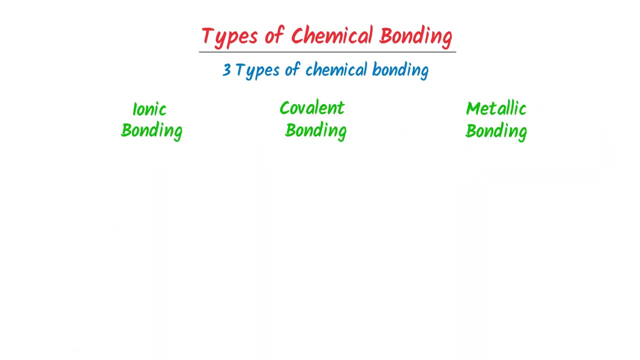 Thus remember that atoms form chemical bond in order to get stability. Now let me teach you the types of chemical bonding. Mainly, there are three types of chemical bonding, like ionic bonding, covalent bonding and metallic bonding. Ionic bonding exists between metals. 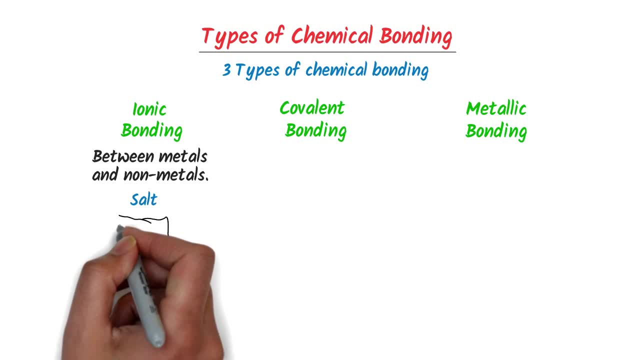 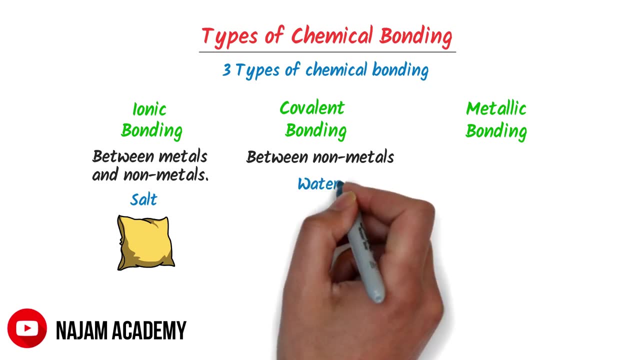 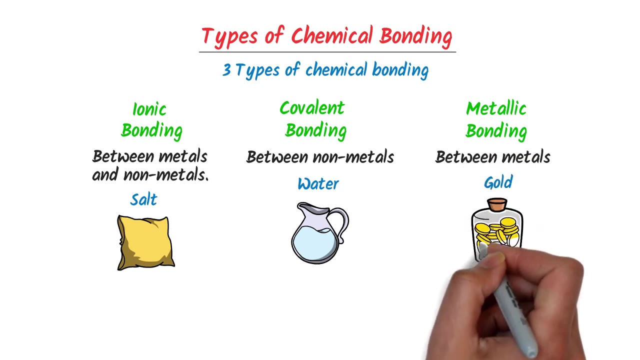 and non-metals, For example, like table salt, sodium chloride, While covalent bond exists between non-metals and non-metals like water, H2O, And metallic bonding exists between metals like gold, iron, etc. To learn more about these types of chemical bonding, watch our lectures.